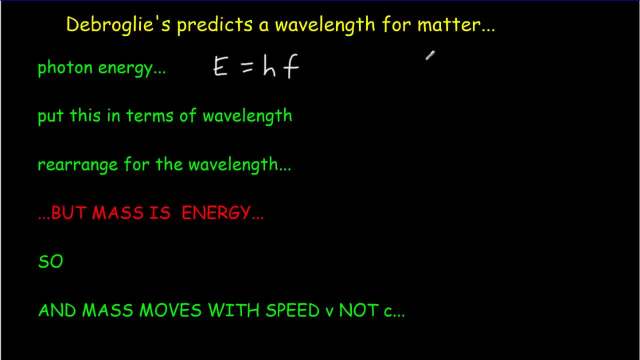 Now we can write that in terms of the wavelength, because we know from the universal wave equation that c is equal to f times lambda, or v is equal to f times lambda, and that means we can write our photon energy as being h times c over the wavelength. 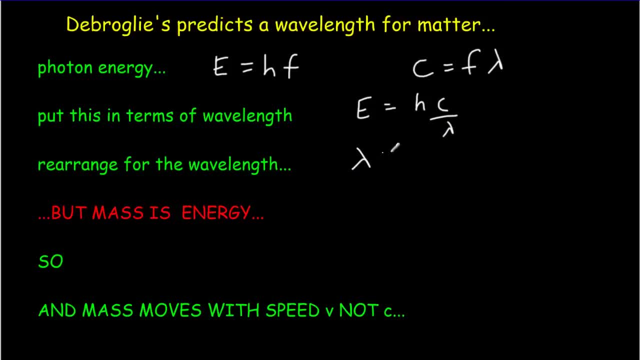 Now, if I rearrange this for the wavelength, I get h times c divided by the energy of the photon. So so far all we've got is an equation for the wavelength of a photon. Now we want to start thinking in terms of mass, and we know there's a relationship between mass and energy. 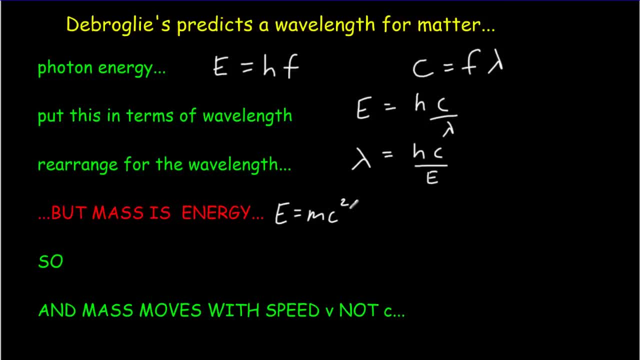 and that is that E equals mc squared, so that we could think in terms of how much equivalent energy would the mass of, say, an electron be, And it would be given by E equals mc squared. So now for our de Broglie wavelength. 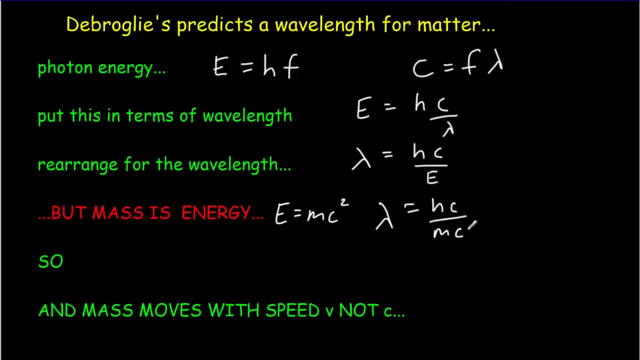 we can put hc divided by mc squared, So we replace photon energy by the equivalent mass energy. And now we make our final step. We can cross out a c or cancel out a c, and then we want to think in terms of m times c. 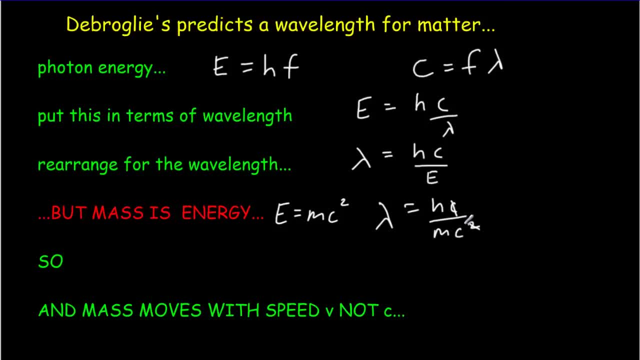 Well, that's mass times, speed of light, but of course we're talking about something with matter, and something with matter won't move the speed of light. It will move at some speed v, which is going to be less than the speed of light. 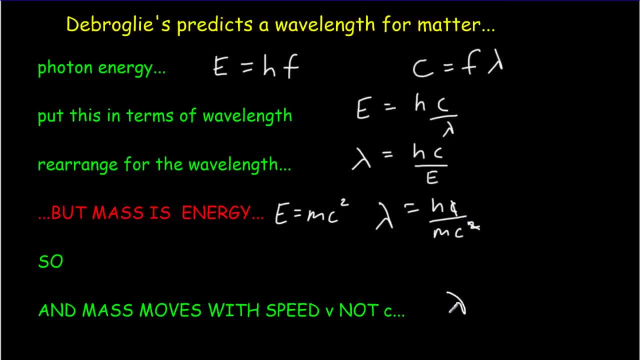 And so if we make that kind of simple substitution, then we get a wavelength for matter equal to h divided by mv, And of course m times v is just the momentum of that particle. So you usually see the de Broglie wavelength written as h divided by p, the momentum of the particle. 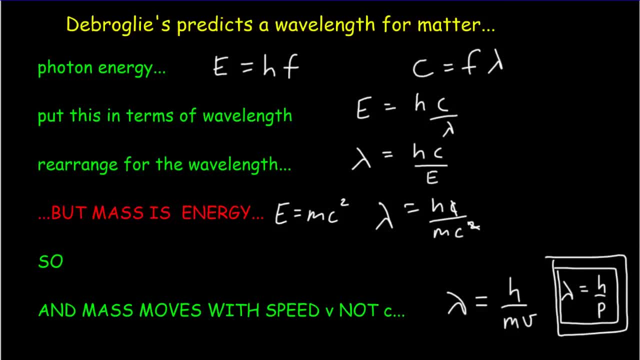 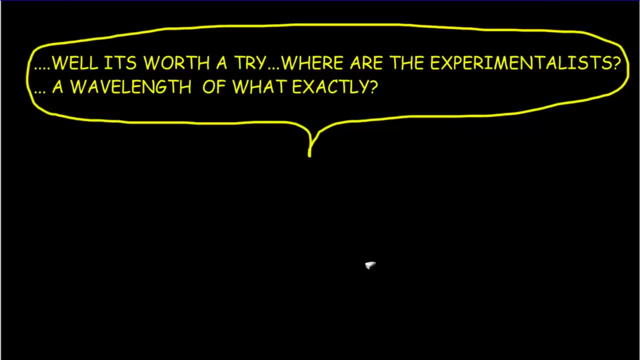 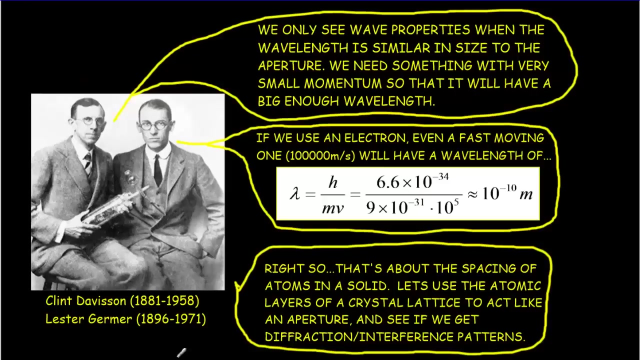 That's our formula for the de Broglie wavelength. So de Broglie makes his prediction for the wavelength and then he issues a challenge out there to all the experimentalists and he says: can you design an experiment so that we can prove that this is really the wavelength of an electron? 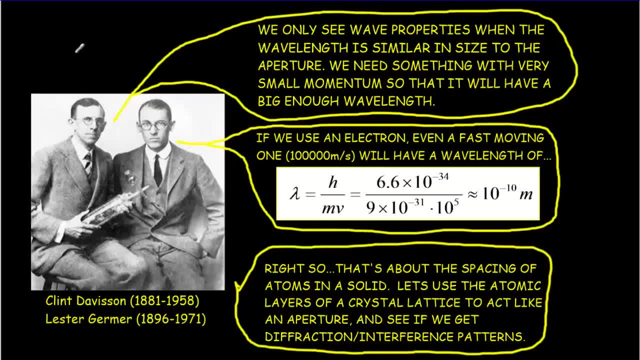 And the two guys that answer the call are Clint Davison and Lester Germer. They know that the primary thing that waves do that particles don't do is interference or diffraction. Particles will not do interference or diffraction. But they also know that the only way that you see interference and diffraction 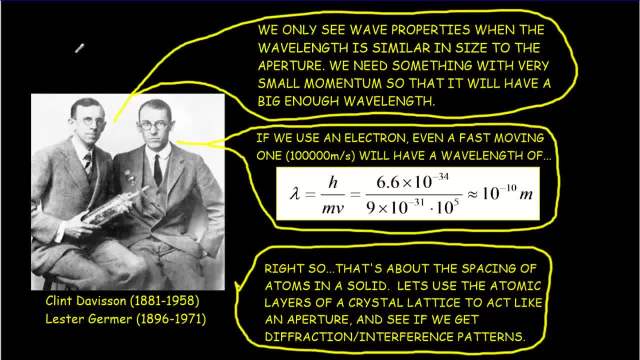 is when the size of your slit, the size of your obstacle, is similar in size to the wavelength. So what they've got to do is use de Broglie's formula and try to calculate what would be a typical wavelength for an electron. 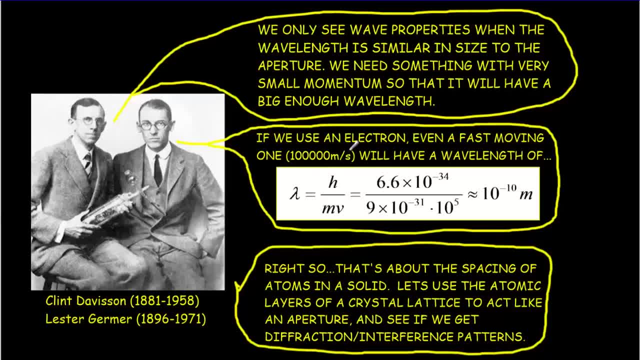 So let's suppose that we- So let's say we- take a fast-moving electron, So let's say it's moving at 100,000 meters per second- We want to calculate what the de Broglie wavelength would be Okay. so he substitutes in: 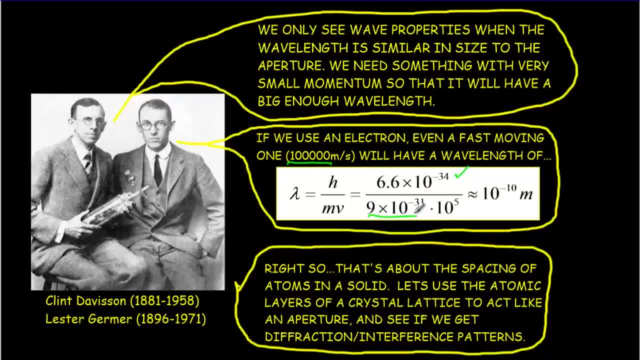 There's Planck's constant, Here's the mass of the electron, That's in kilograms, And this would be the speed of the electron in meters per second. Do that calculation and you get an answer of about 10 to the minus 10 meters. 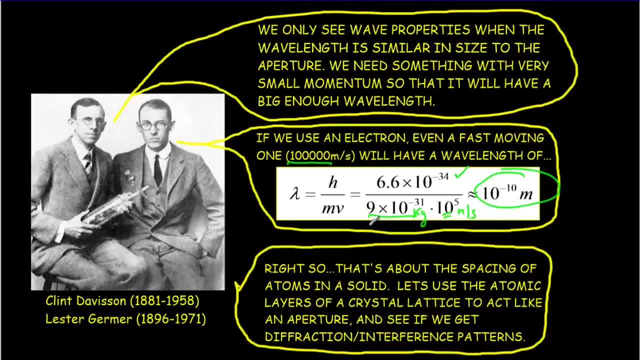 So they're thinking: okay, well, what in the real world is? an electron has a size of about 10 to the minus 10 meters, And hopefully you're aware of the fact that the size of an atom is about 10 to the minus 10 meters. 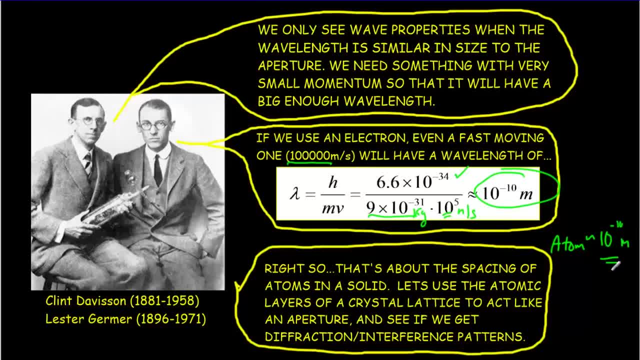 So this is one of those orders of magnitudes that you're supposed to remember in this course. So remember an atom- 10 to the minus 10 meters, A nucleus about 100,000 times smaller, or five orders of magnitude smaller, at 10 to the minus 15 meters. 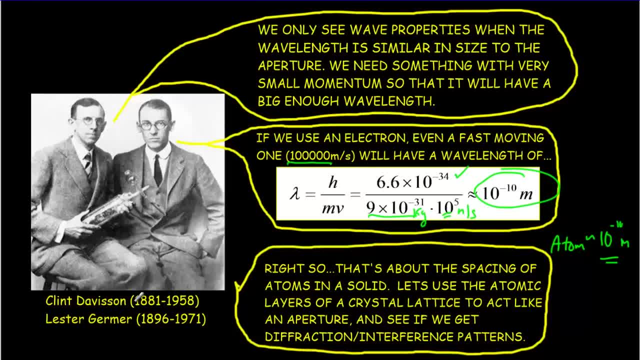 So their idea is we're going to send some electrons onto a crystal, because the atoms are going to be separated by about 10 to the minus 10 meters, And so they'll kind of form a diffraction grating and we should be able to get some sort of diffraction pattern. 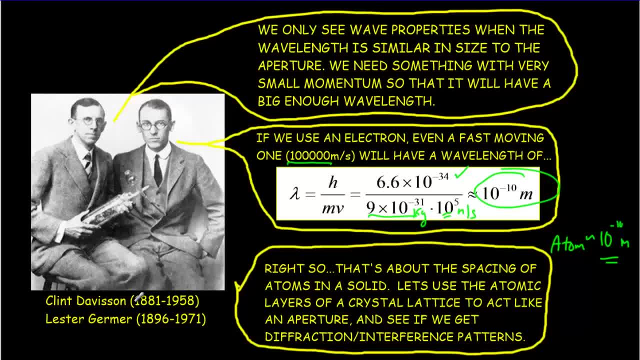 And of course, the primary thing that you see when you've got a diffraction pattern is you'll see places where the electrons show up and then the intensity really drops and then the intensity comes back up again. So the intensity will go up in certain places, drop down. 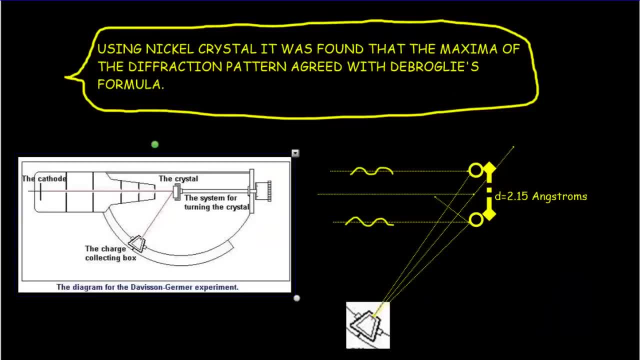 and come back again. Particles never do that, but waves do. So what they did was they used a nickel crystal. they fired the electrons at it, so they accelerated the electrons through a voltage, sent lots of electrons onto this crystal here. 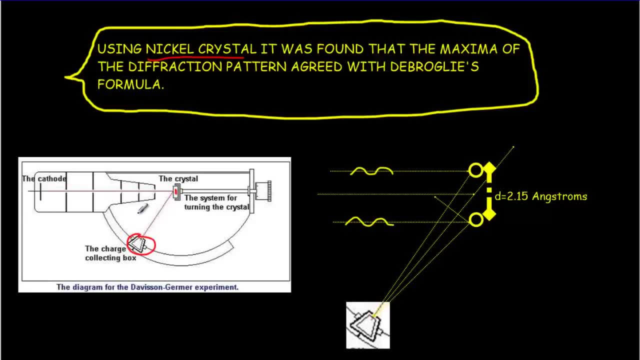 and then they had a detector over here and this detector would register the number of electrons that are hitting as this angle here is changed. Now I don't want to go into the geometry of this very much, but you can imagine you've got two nickel atoms right here. 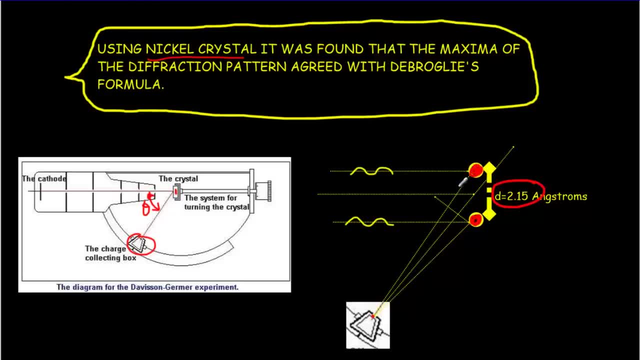 They have a certain spacing between them and waves would come in and reflect off those atoms And the waves reflecting off the atoms could interfere with each other. And so, once again, if you can fit an integral number of wavelengths into that path, difference. 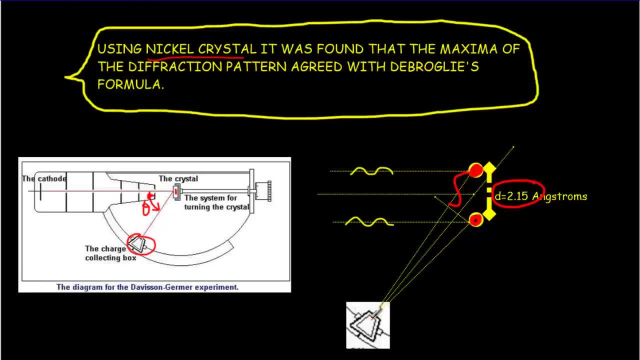 then you're going to get a pattern of constructive interference, And that would mean, if this is equal to an integral number of wavelengths, you're going to get a high intensity at that particular angle here, Of course, as you veer away from that angle. 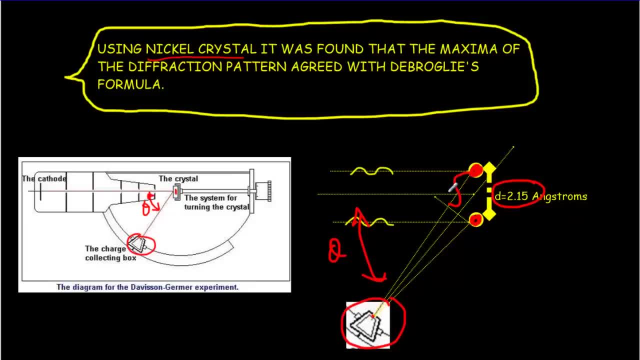 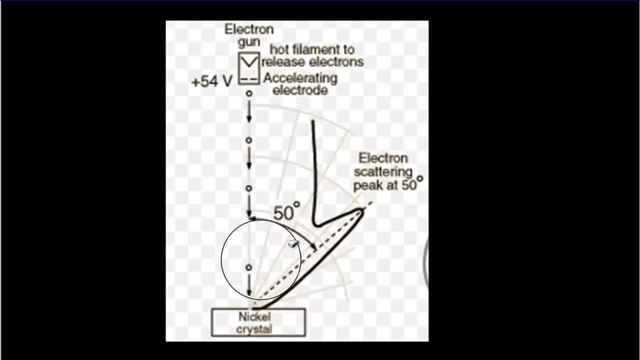 then the path difference will no longer be at one whole wavelength and you won't get that perfect constructive interference and the intensity is going to drop off. So this is what their data looked like. They got a peak right here at an angle of 50 degrees. 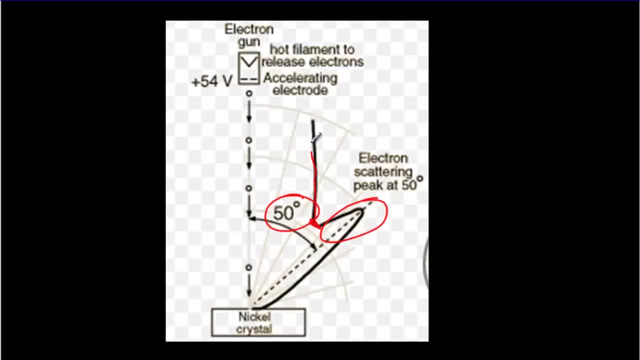 And then the intensity it drops off and then it comes back again, And that's a diffraction pattern. And when they did all their calculations they found out that the de Broglie wavelength exactly predicted that the maximum would occur at 50 degrees. 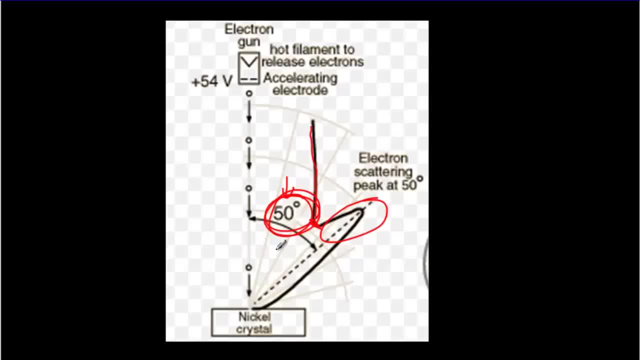 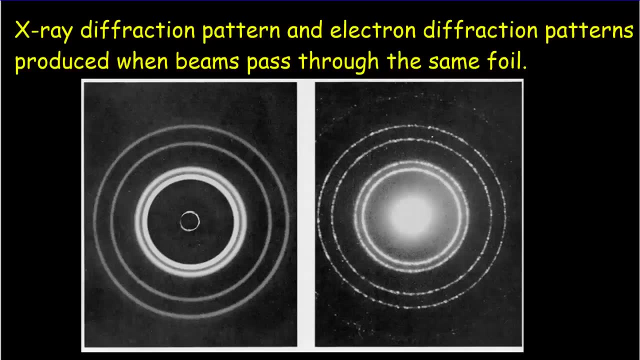 So Davison and Germer not only showed that you've got a diffraction pattern, they verified that the de Broglie wavelength was correct. What you're seeing below is two images: One is made with X-rays and the other is made with electrons. 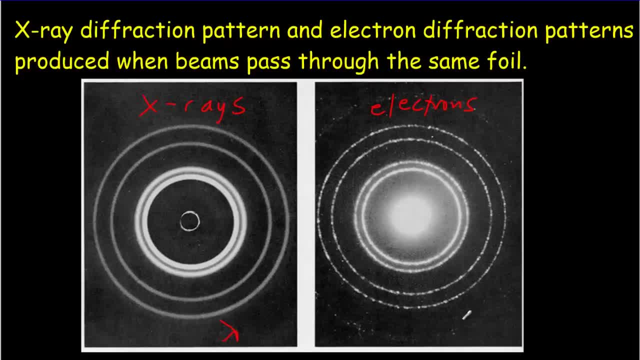 But the wavelength of the X-rays is exactly the same as the de Broglie wavelength of the electrons. So these two wavelengths are the same And what you're seeing here is an interference or diffraction pattern. So, for instance, right in here you're not getting any X-rays. 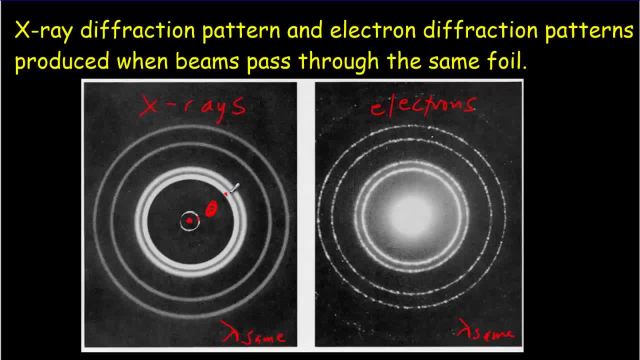 And then you're getting lots of X-rays and then no X-rays and lots of X-rays, no X-rays, lots of X-rays, etc. And same pattern with the electrons, And you're seeing the high intensity places occurring at exactly the same places. 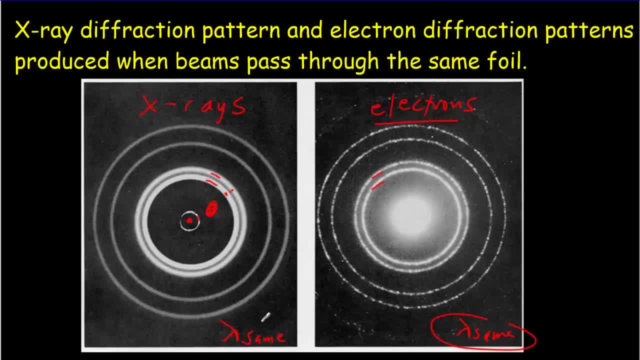 for the electrons as for the X-rays, And that's because the wavelengths are the same. So right here we're getting lots of electrons then no electrons, lots of electrons, no electrons then lots of electrons, none, etc. So only waves can do this. 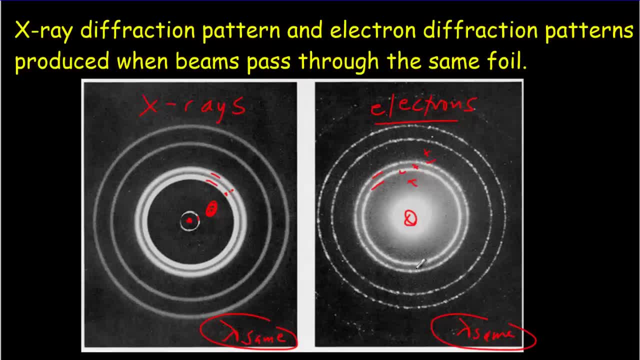 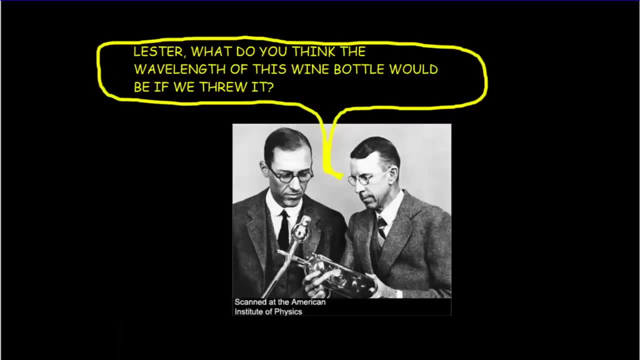 Particles in themselves can't do it, but particles exhibiting their wave nature can do this type of diffraction pattern. Okay, we've got this de Broglie wavelength. What happens when we look at the de Broglie wavelength of, say, a macroscopic object? 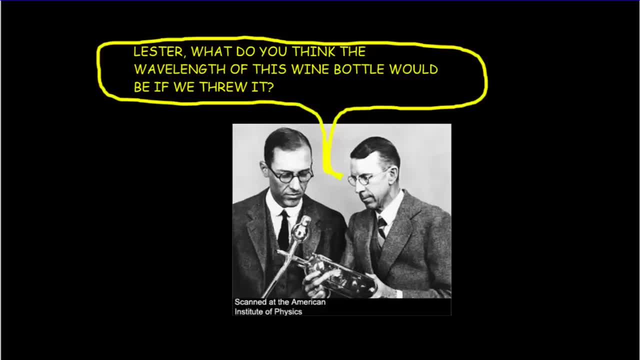 like a baseball or, in this case, a wine bottle. And in this case it's not really a wine bottle. This is actually their experimental apparatus here. So the wavelength is going to be given by Planck's constant, divided by the momentum. 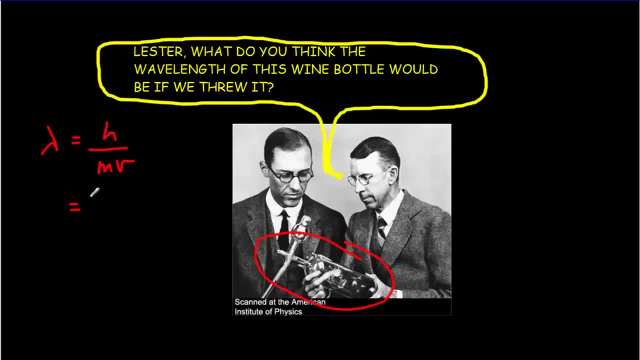 which is the mass times the speed. So we've got to make up a mass and make up a speed for our wine bottle. Let's take nice simple numbers. Let's say that the mass of the wine bottle is about 1 kilogram. 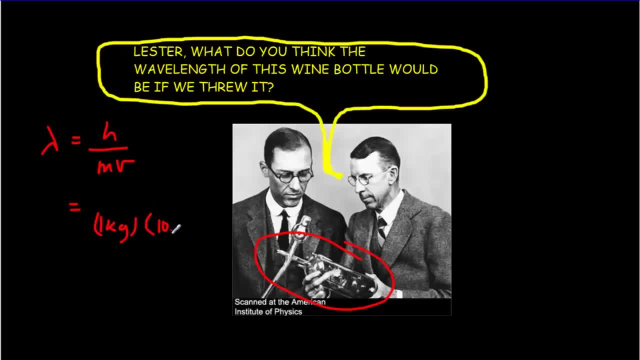 And let's say we throw it at 10 meters per second, Of course, Planck's constant is 6.63 times 10 to the minus 34 joule seconds, And so we're going to get an answer of about order of magnitude of about 10 to the minus 35.. 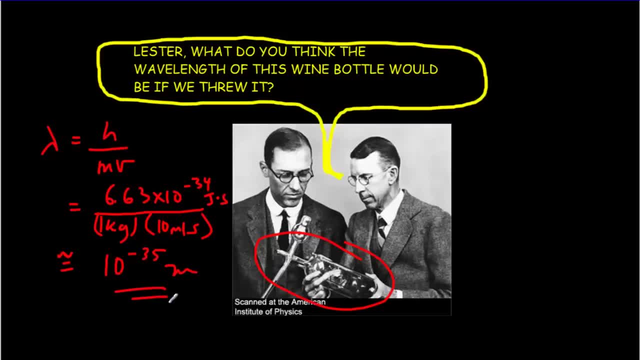 Meters 10 to the minus 35 meters is a small number. In fact, there's nothing that we know of in the universe that is that small. We're never going to get diffraction effects or interference effects on macroscopic objects. 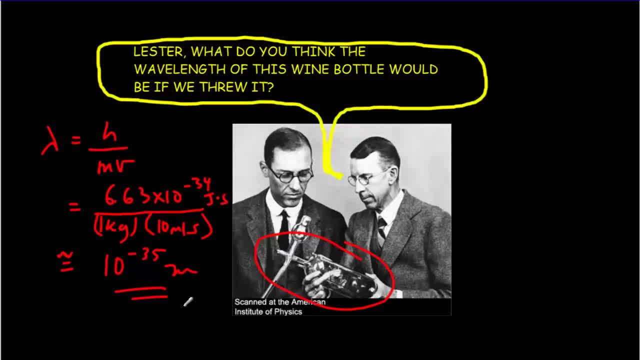 It's just going to happen for subatomic particles, So you don't have to worry about, let's say, you're walking through a door. You don't have to worry that as you walk through that door you're going to diffract. 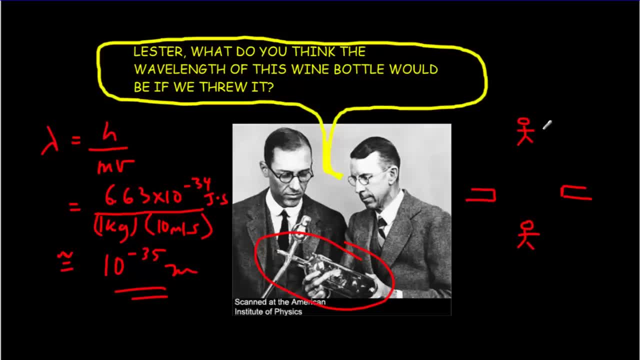 And some of the time you're going to get diffraction, You'll go straight through, But other times you'll end up over here or maybe over here. You'll never end up over here or over here. So, anyways, you don't have to worry about that. 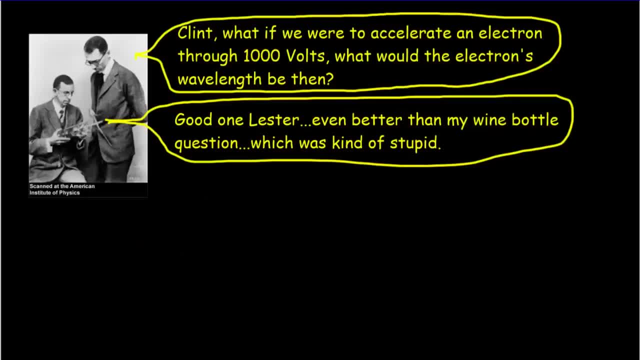 That's not going to happen for macroscopic objects. Now, typically, the type of objects that you're dealing with is electrons, And you accelerate them through some voltage. So a meaningful problem- and a problem that often comes up in the IB- is to calculate the 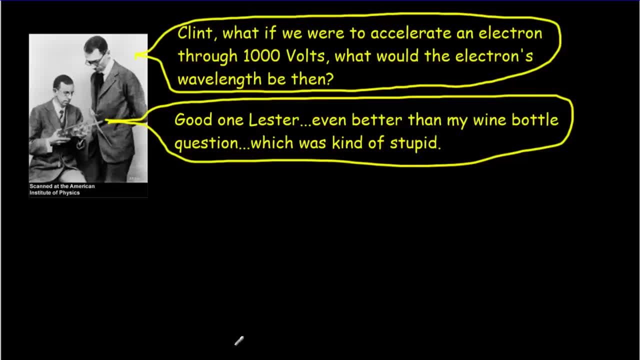 wavelength of an electron when it is accelerated through a given voltage. So the type of energy transformation that we're talking about is going to be a loss of electric potential energy as that electron gets accelerated across the plates, And it's going to result in a gain in speed or a gain in kinetic energy for that electron. 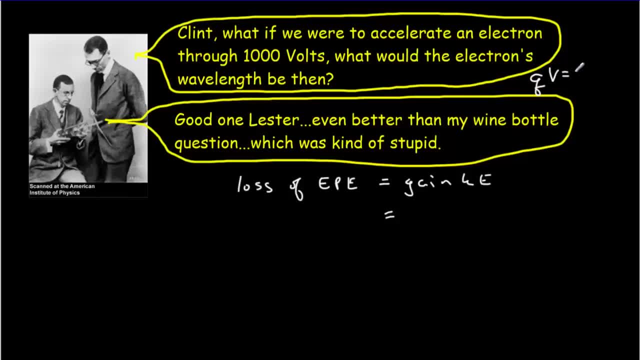 So it's really- We're really just going to use QV equals work, But the work is going into changing the kinetic energy. So our gain in kinetic energy- assuming it starts from rest- would be a half mv squared. I'm going to write that as p squared over 2m. 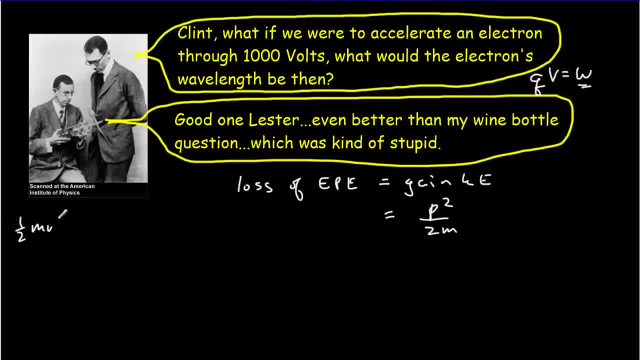 Now, if you're not familiar with a half mv squared being equal to p squared over 2m, what you have to do is remember p is equal to mv. So then if I square both sides, I'll get p squared equals m squared times v squared. 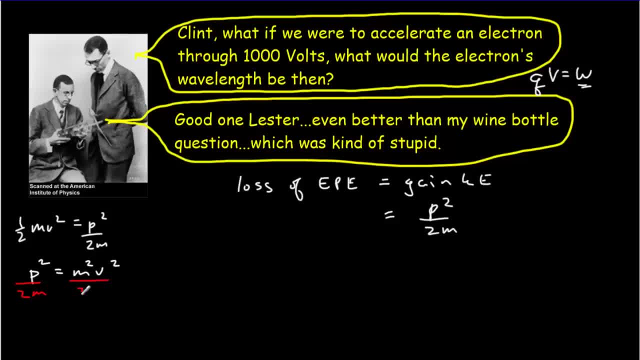 And then if I divide both sides by 2m, then m will cancel out and I'll get a half mv squared. So a half mv squared, or kinetic energy, is the same as p squared over 2m, And that is in your data booklet. 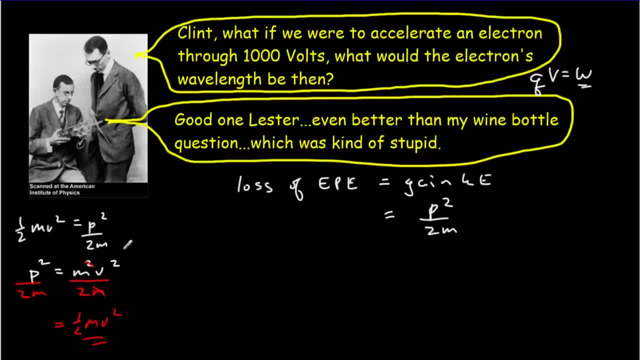 Now the loss in electric potential energy is just going to equal the charge. in this case it's the charge of an electron accelerated through a voltage v. Now the next thing that we want to do is we want to get rid of that momentum. 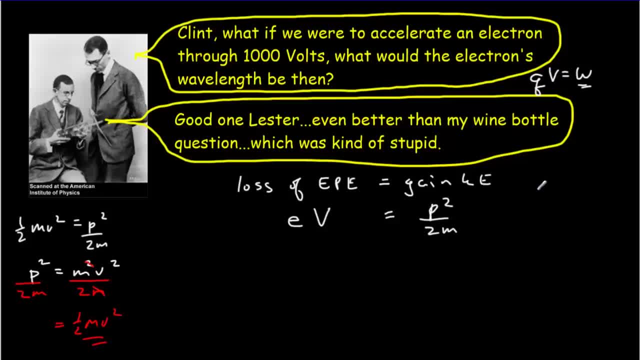 And put it in terms of the de Broglie wavelength. So we know. the relationship is that the de Broglie wavelength is equal to h over p, And that means that p is equal to h divided by lambda, And that's what we're going to substitute in here for p. 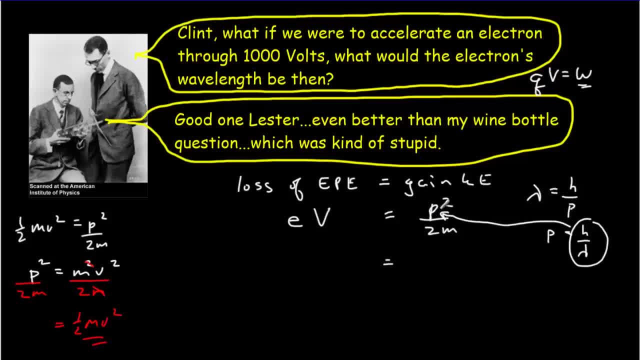 So we make our substitution. We replace p by h over lambda. So p is going to become h squared divided by lambda squared, And then we'll have a 2m on the bottom And that will equal e times the voltage. Now let's rearrange that for lambda. 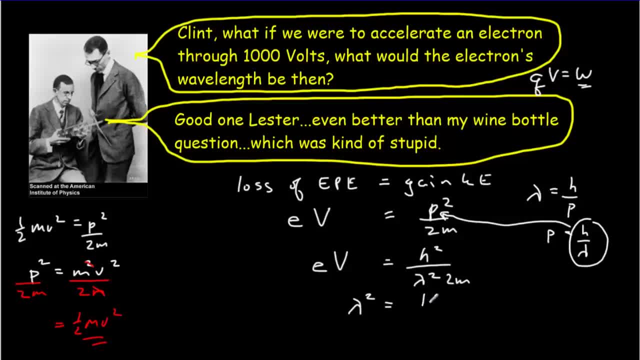 Lambda squared will be equal to h squared all over 2m times ev. Taking the square root of both sides, we'll get that lambda is equal to h all over 2m ev square root. Okay, so let's substitute the numbers in and see what we get for our wavelength. 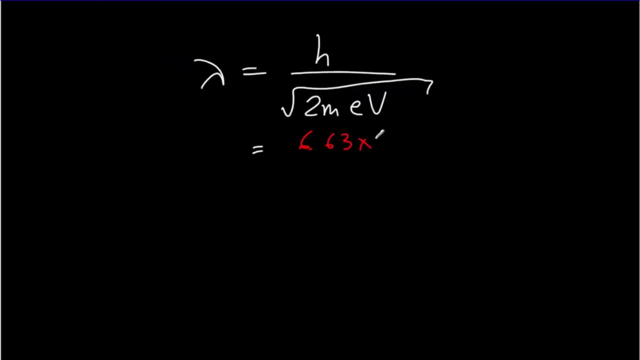 h is 6.63 times 10 to the minus 34.. That would be joules times seconds. And then we've got to divide that by the square root of all these numbers too. Mass of an electron. you can look that up in your data booklet. 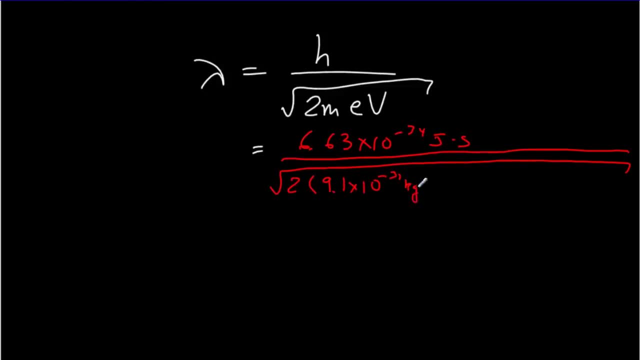 It's 9.1 times 10 to the minus 31 kilograms, Times the charge of an electron, 1.6 times 10 to the minus 19.. And that's in coulombs, And the voltage we were accelerating. 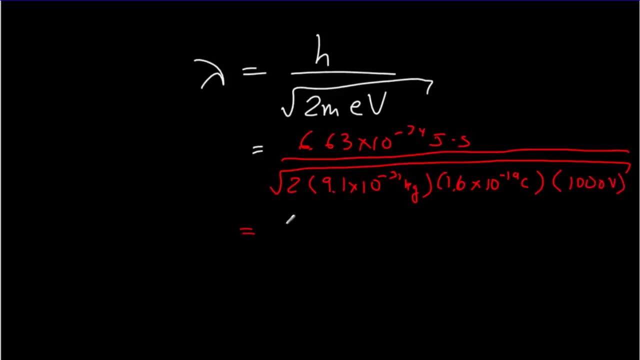 We're putting it through is 1000 volts, And if we multiply that all out we should get an answer of 3.9 times 10 to the minus 11 meters. So we're talking once again of the order 10 to the minus 10 meters. 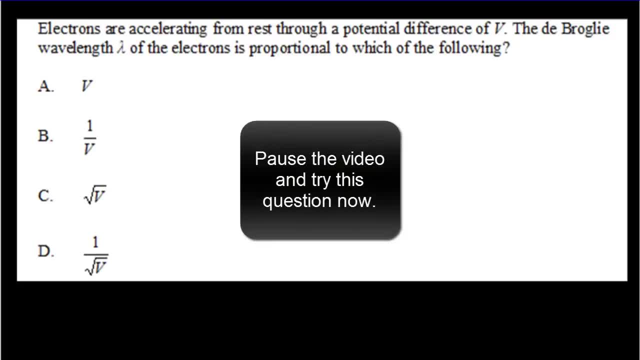 if we accelerate through 1000 volts? Okay, a few IB questions. Read over the question, try it out and then come back for the answer. Okay, so in this one we've got the same voltage velocity, But we come back to that equation we just derived. 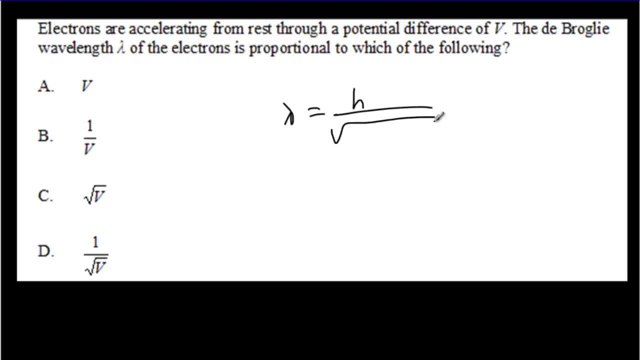 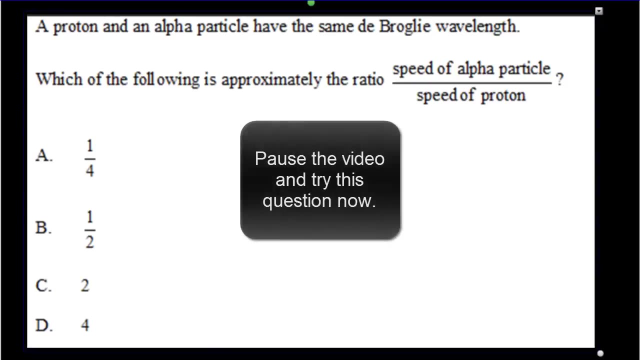 We know that eseq another IB question. we're taking over cities and talk about him in combat for the answer. We've got the same de Broglie wavelength. If we have the same de Broglie wavelength, of course the de Broglie wavelength is given by h over p. 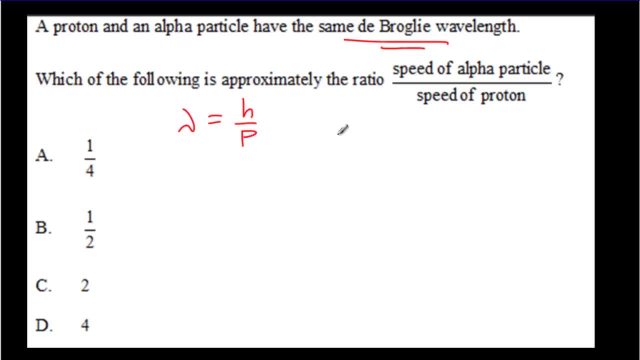 h is a constant, so that means that our momenta must be the same. So that would mean that the mass of the proton times the speed of the proton must equal the mass of the alpha particle times the speed of the alpha particle. Now, an alpha particle, it's got two protons and two neutrons, so it's got four nucleons in total. 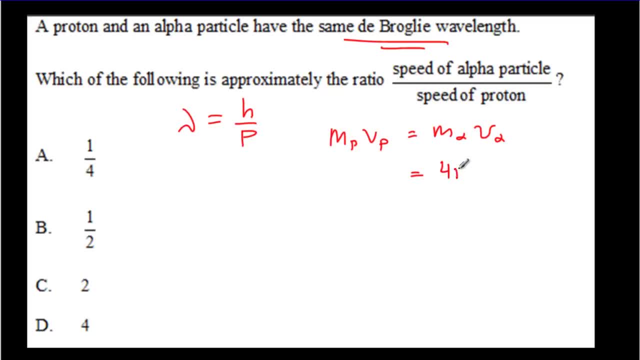 So we can say that it's got four times the mass of a proton or a neutron, whereas over here we've just got the mass of the proton And we're looking for the ratio of the speeds, So the speed of the alpha particle divided by the speed of the proton. 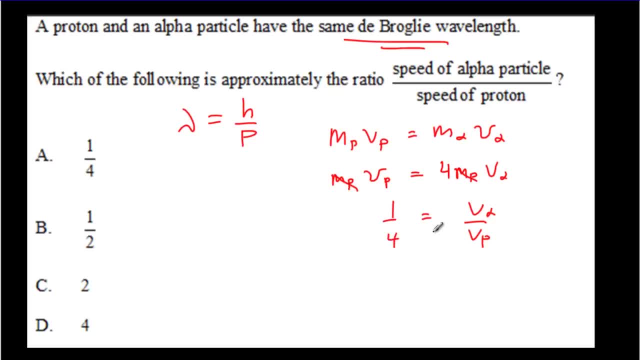 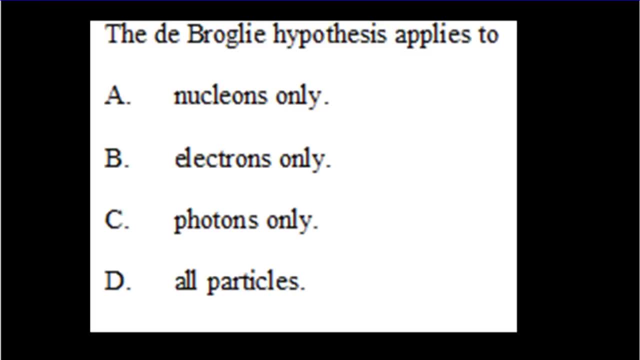 we can cancel out those masses is going to equal 1 over 4, and that means the correct answer is answer A. Another IB question. read it over, try it out and then come back for the answer. So the de Broglie hypothesis. so the correct answer here is D. 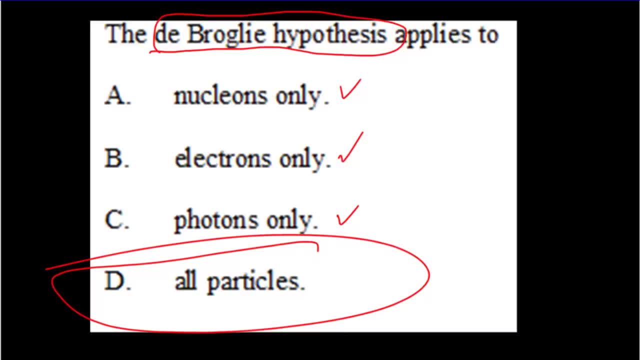 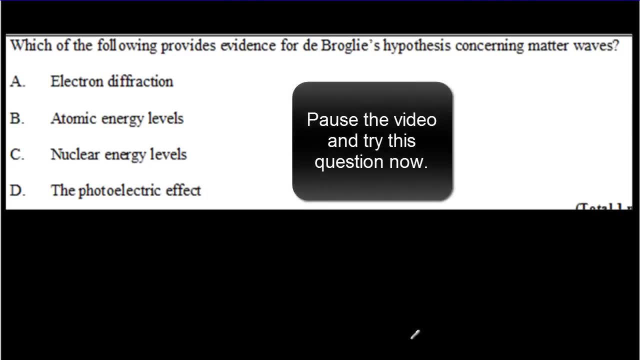 It can even apply to baseballs. it's just that there's nothing small enough in the universe so that the baseball could show its wave nature and diffract. One more IB question. read it over, try it out and then come back for the answer. 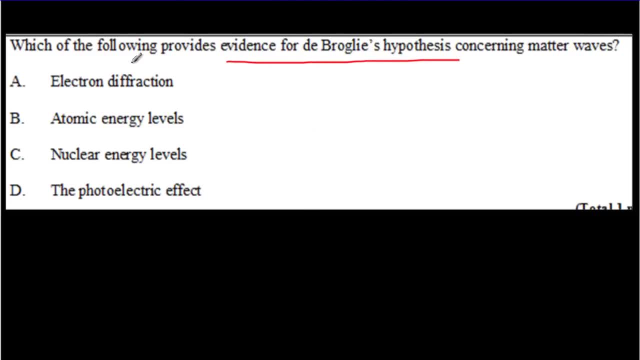 Okay, what provides evidence of de Broglie's hypothesis? Well, that would be the electron diffraction. whether it's electron diffraction of a nickel crystal, or it could be off a thin metal foil, If we're getting electron diffraction patterns. 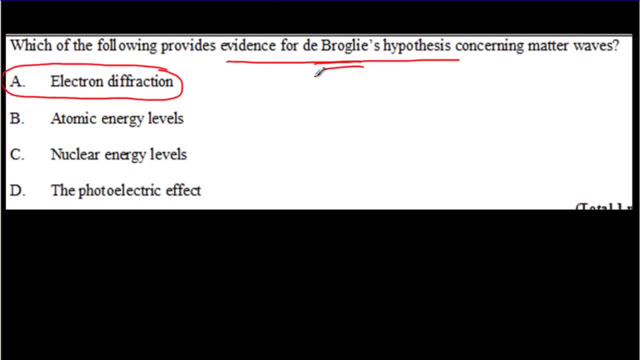 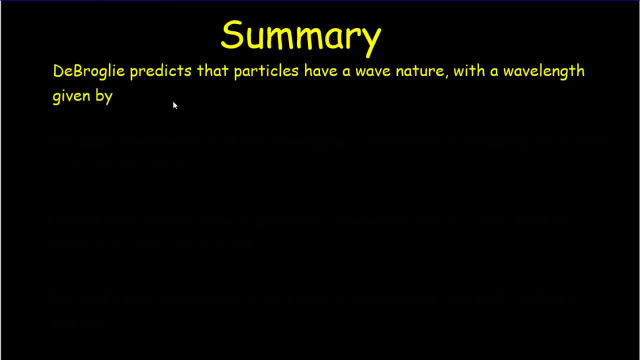 that's evidence of de Broglie's hypothesis that matter has a wavelength and a wave nature. Okay, so let's summarize what we've said. First of all, de Broglie predicts that particles do have a wave nature and the wavelength that we'll describe.